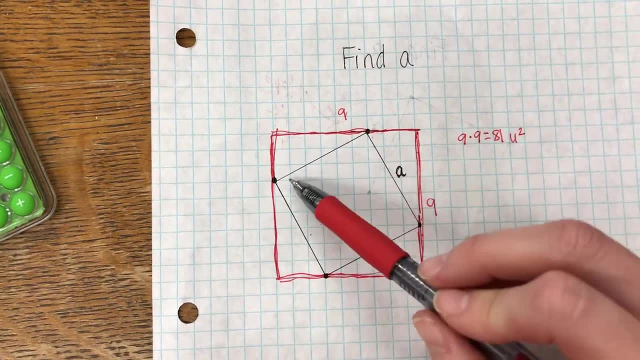 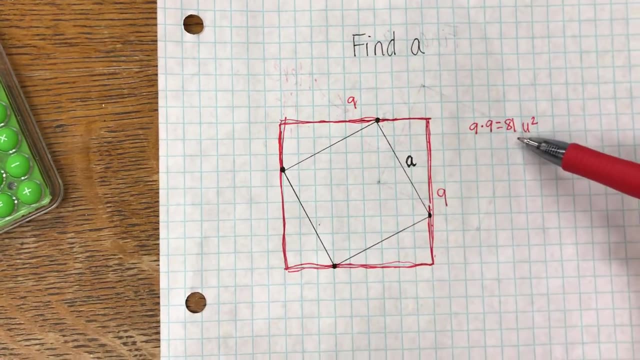 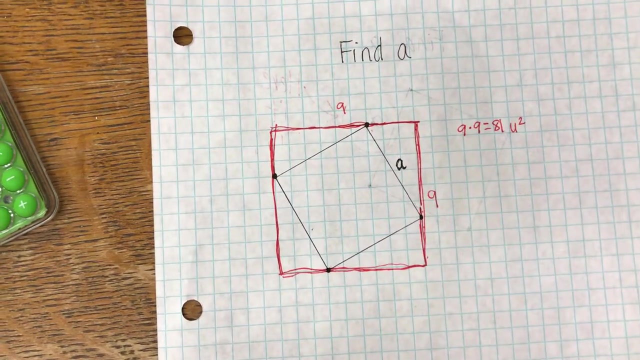 I actually need. I know this smaller square inside is not 81 units. I've got all this extra space that I don't need, so I need to get rid of that extra space. take it out of the 81 that I've already counted. so to do that, I have to figure out what is the area of these triangles. 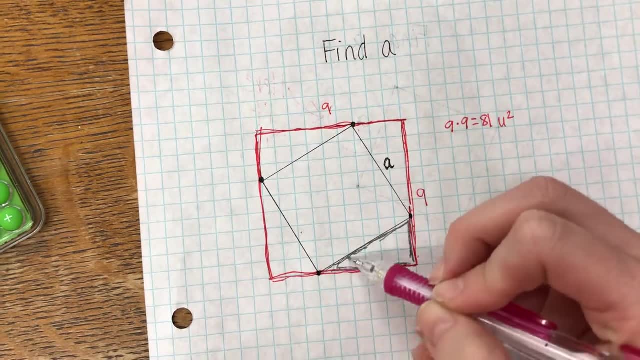 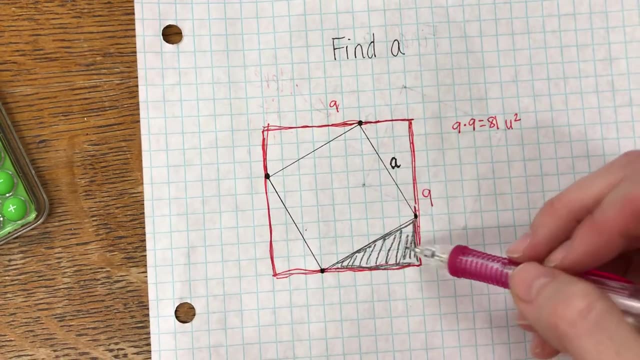 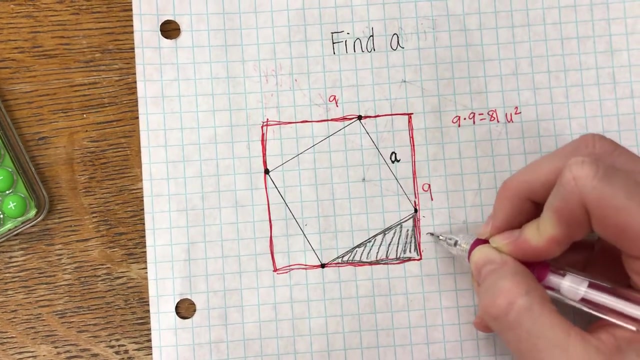 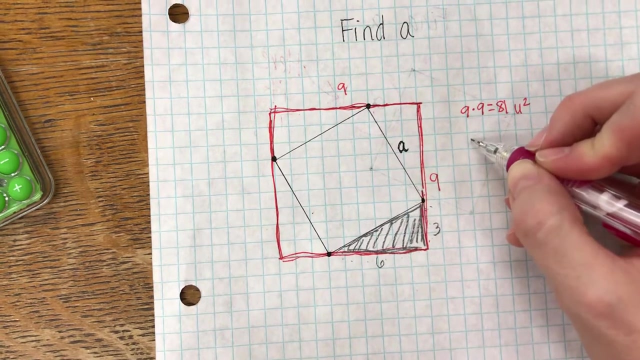 that are on the outside. once I know what those triangles equal, I can subtract them from the 81 of the big square and whatever is left is going to be this little square here. so this triangle is one, two, three, four, five, six, and hopefully you remember that the area for a triangle is 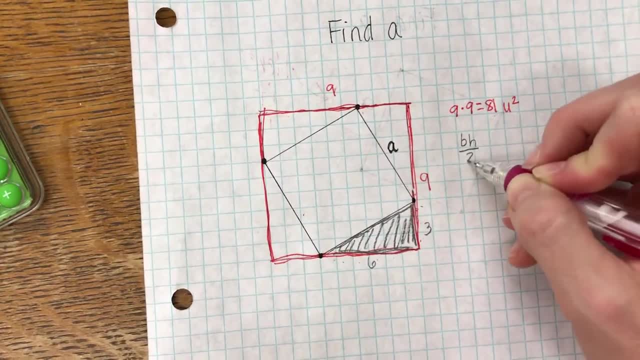 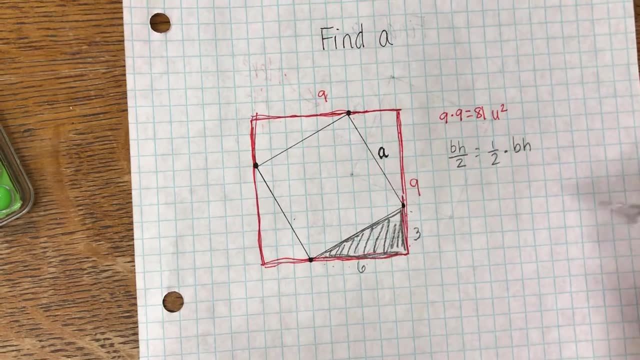 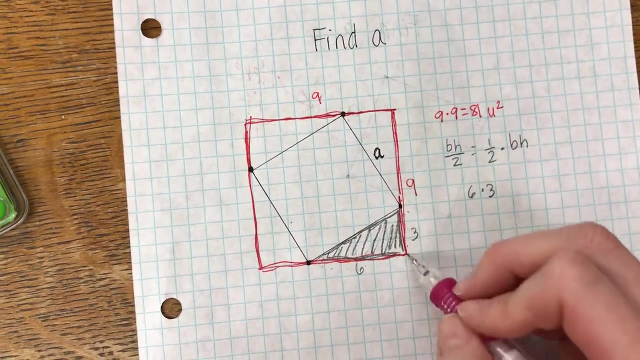 calculated by base times height divided by 2 or 1 half times base times height. you can see that written a couple of different ways. so this triangle is 6 times 3. the base is 6, the height is 3. divide that by 2. I have 18 divided by 2. 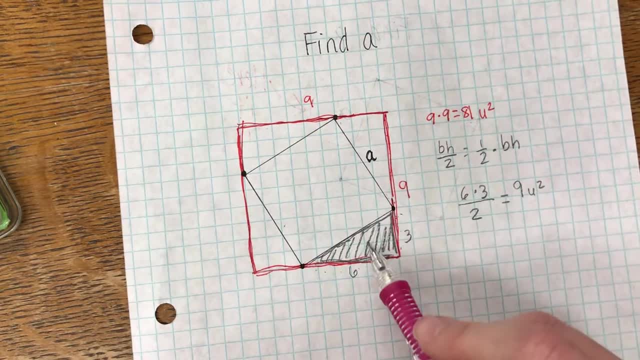 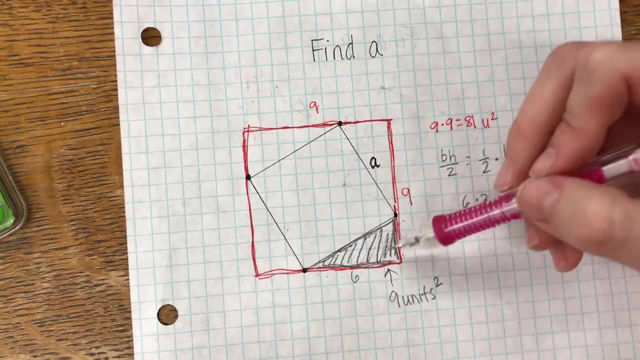 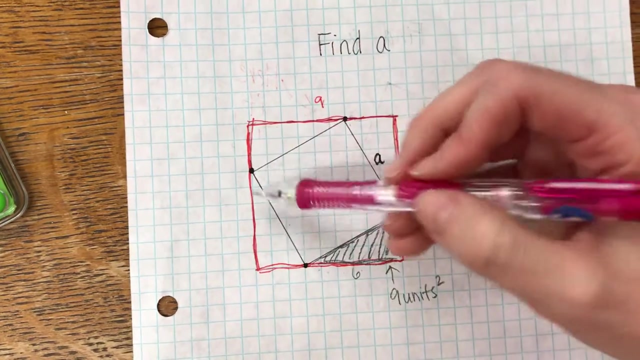 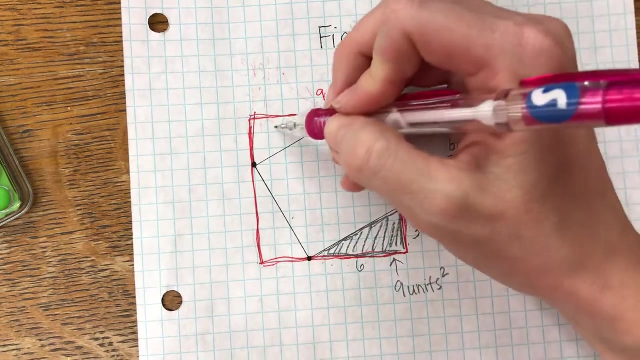 divided by two is nine. so one triangle is nine square units and I have four triangles like that. they're all the same triangle. this one is three by six, this one is six by three, six by three, so they have the same dimensions. this nine units is going to be the size of this triangle and this triangle and this triangle. so 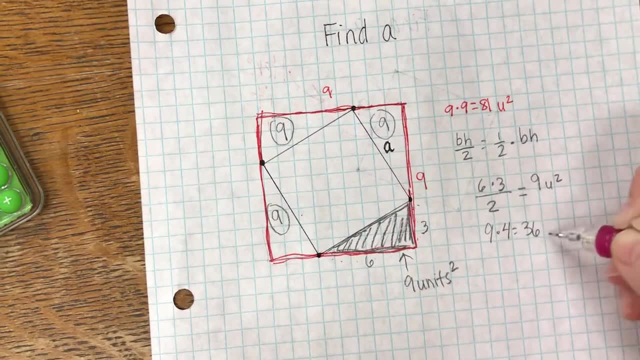 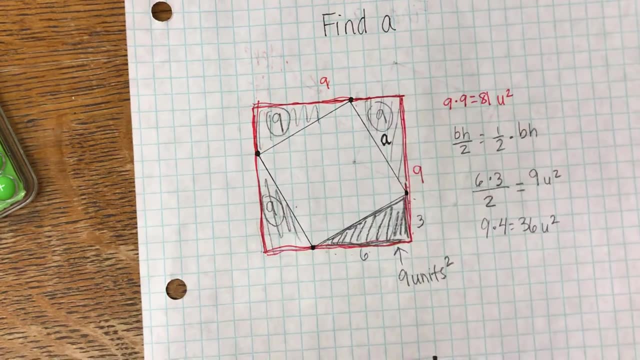 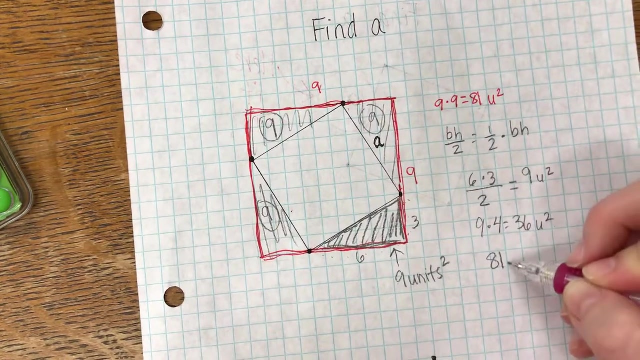 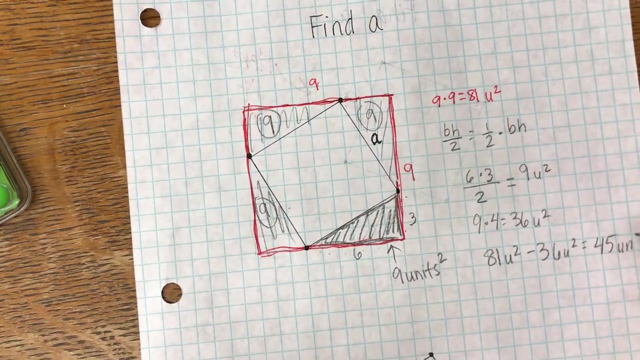 nine times four is 36 square units. that's the area of all these triangles that I don't want. so my large square of 81, minus the triangles of 36 that I didn't want, equals 45 square units. so the area of this square is: 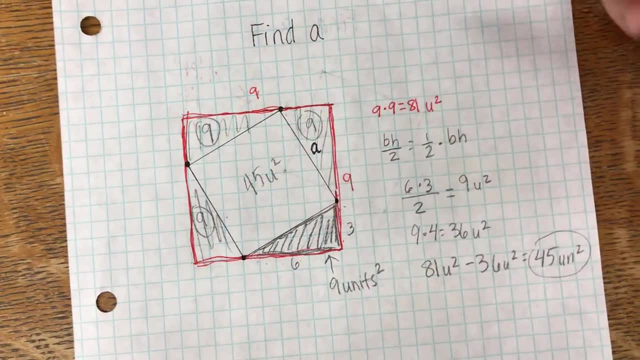 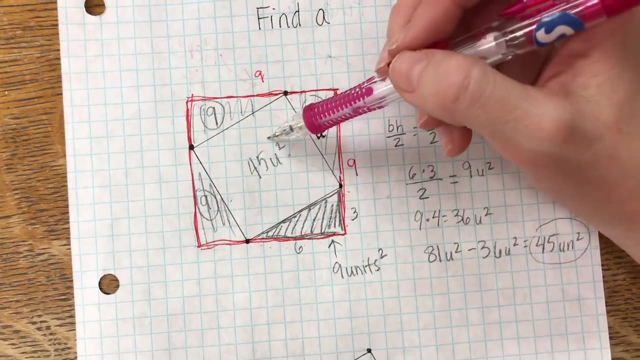 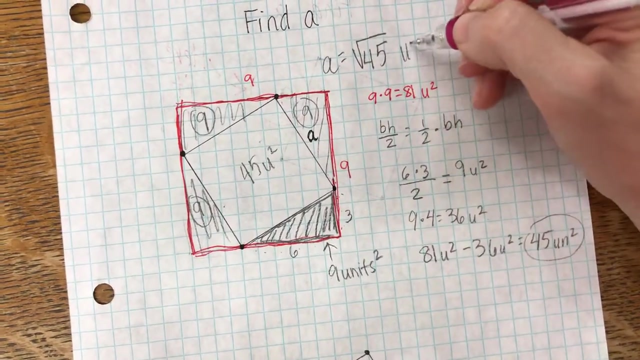 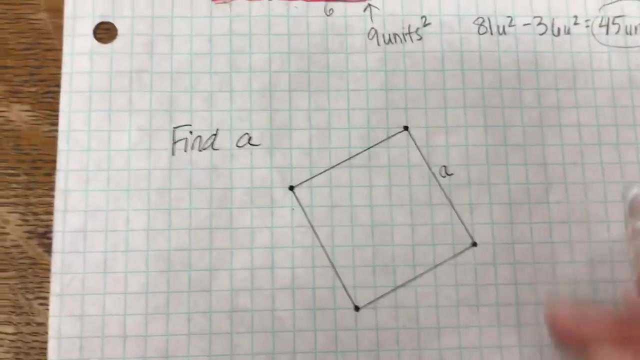 45 square units and we've discussed how the side length of a square is just the square root of the area, so in this case, a would equal the square root of 45 units. the other strategy is to separate the square into pieces inside of the square and then find out what the square is and then find out what the square is. 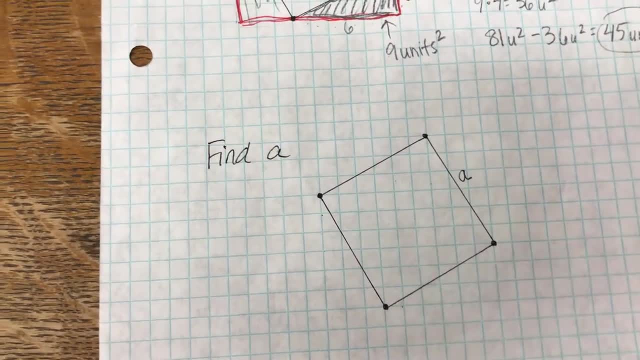 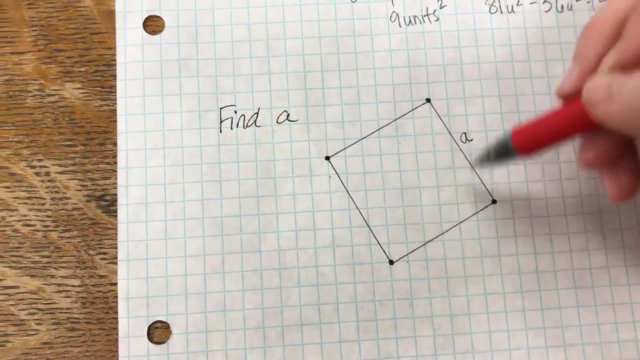 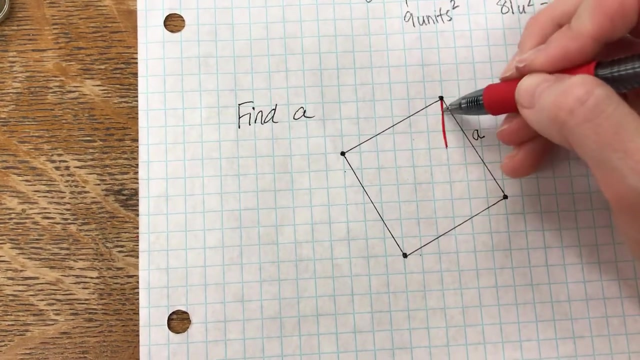 and then find out the pieces that are inside and add them all together. so one way to do that would be to look for rectangles or triangles that you could find the area of. I'm gonna split this one into a triangle. well, a couple of triangles I see, if I come straight down and go straight over. 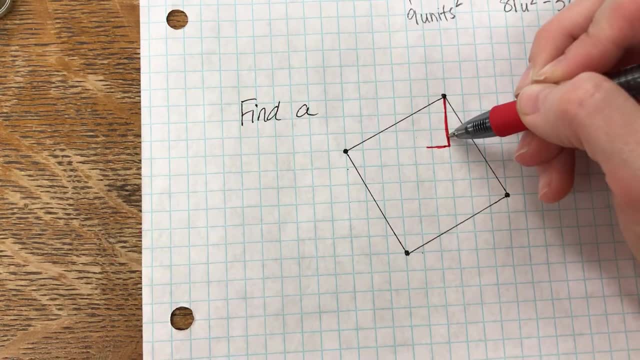 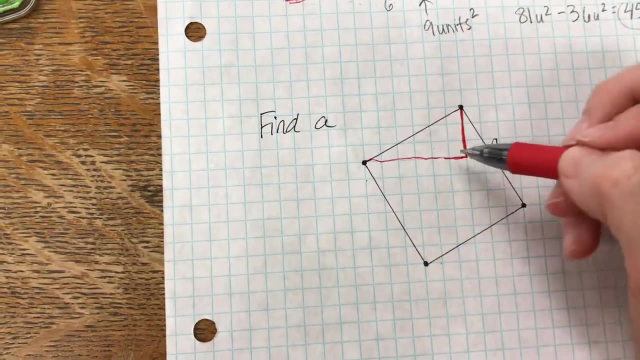 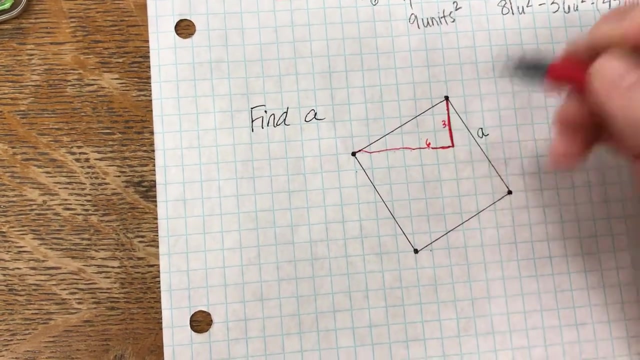 I have a right angle and that's nice. I can figure out a base and a height to make the triangle that's well knit diagonal that we just cut off. it doesn't have to be, or it'll tear right, but that's fun. really easily to find out the area of this triangle: 1, 2, 3, 4, 5, 6 by 3, 6 times. 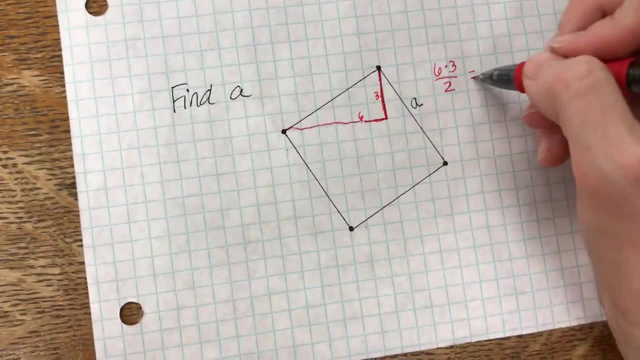 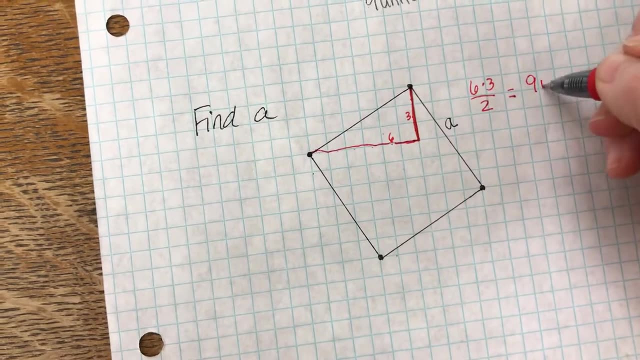 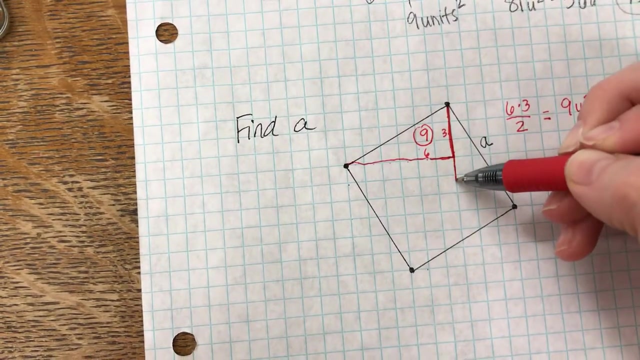 3 divided by 2 is like we had up here 6 times 3 divided by 2. it just happens to be the same triangle is 9 square units, so this triangle is 9. then let's see, if I keep coming straight down, I'm gonna turn my paper. actually I don't want to. 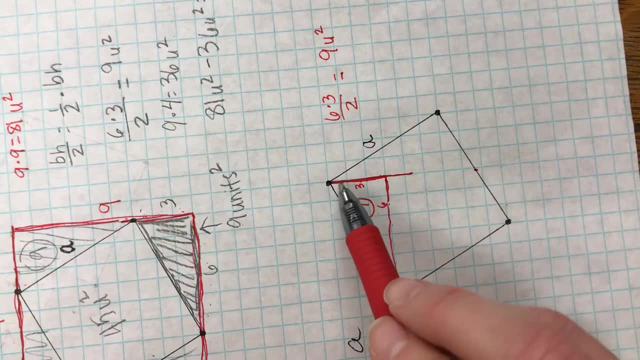 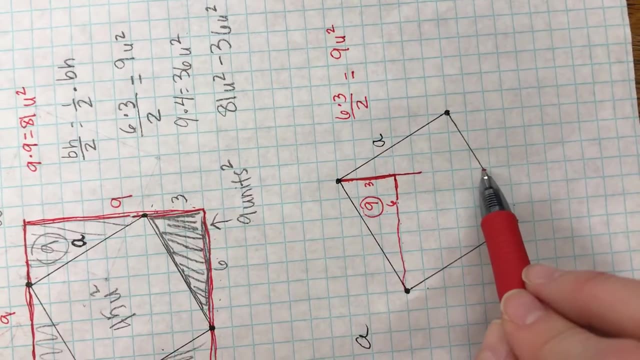 come all the way over to the edge, because when I go to count a base- 1, 2, 3, 4, 5, 6, 7- I don't really know how much that is. I would just be estimating and I don't want to do that. I want to be precise. so I'm gonna go to here and go. 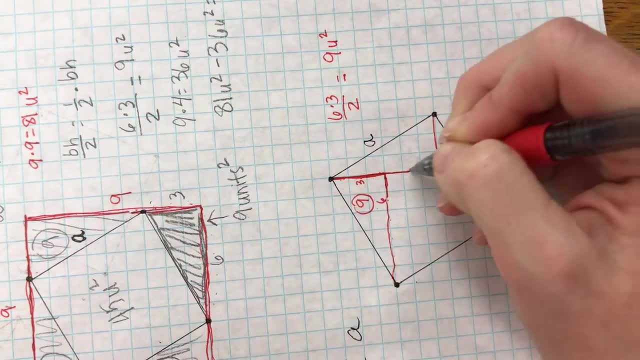 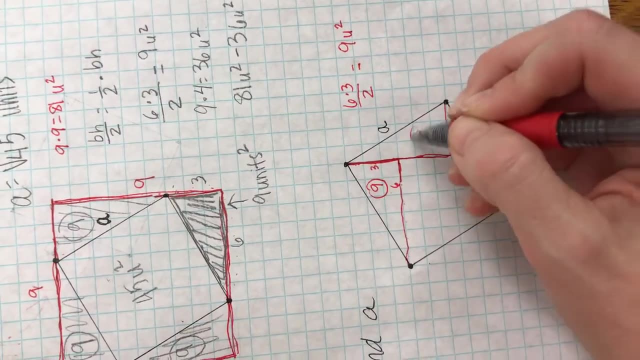 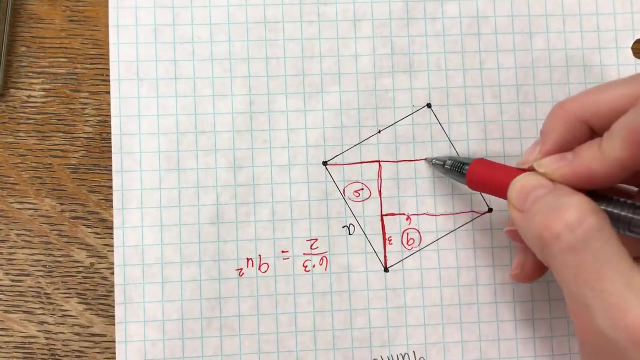 straight up. so actually this triangle is just like the one I just calculated: 3, 2 by 6, so this area is also 9. then I can do the same thing over here again. I don't want to go all the way to the edge, but I can go to where I have a straight.